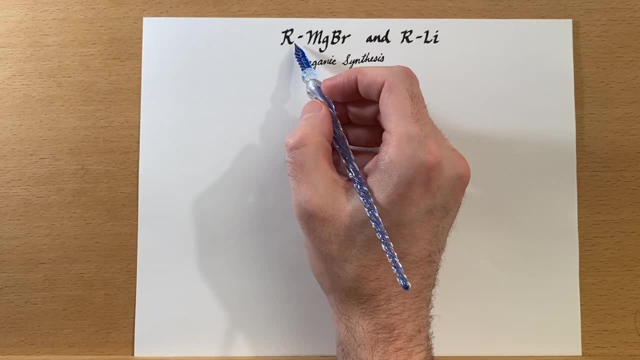 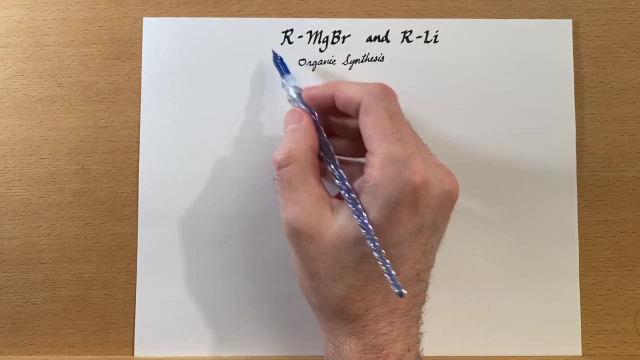 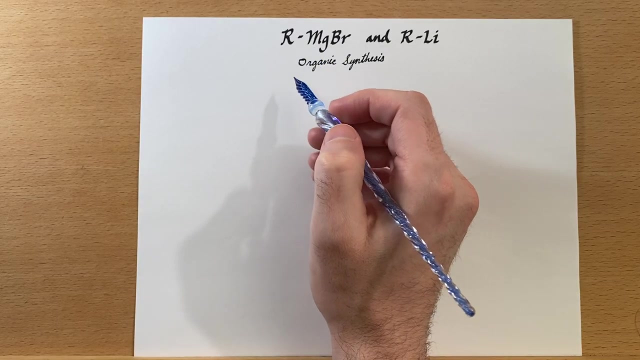 We're really only limited by the fact that we can. We can't have a carbonyl contained within this R group, or an alcohol or any kind of protic material here, But beyond that there's quite a bit of those that we can make. 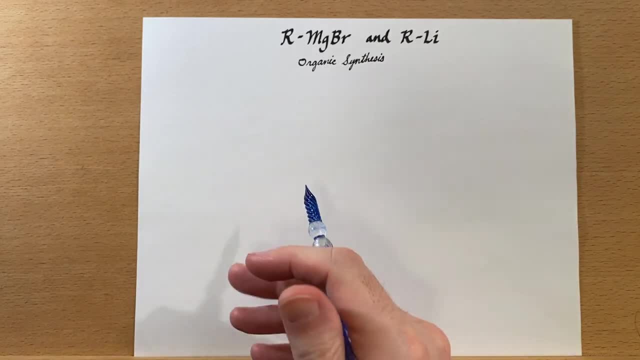 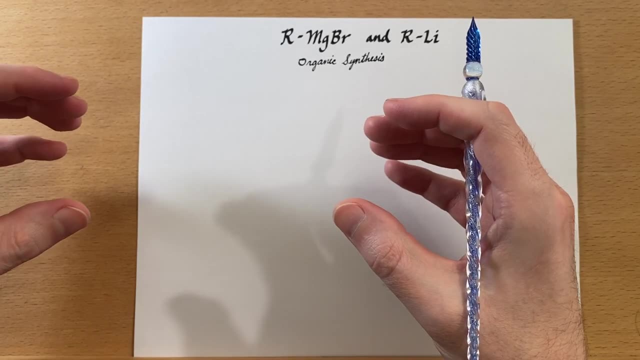 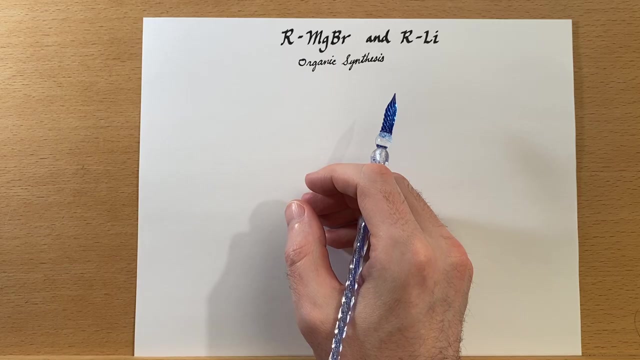 And these are quite important when we're trying to make a carbon carbon bond, And what this allows us to do is start with smaller pieces of the molecules that we're looking to build and start putting them together. This can greatly enhance our yields and flexibility in synthesis. 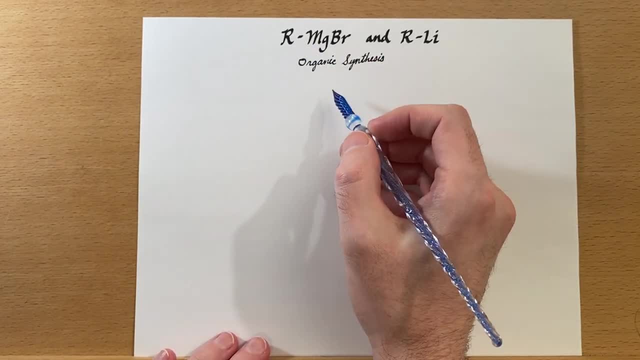 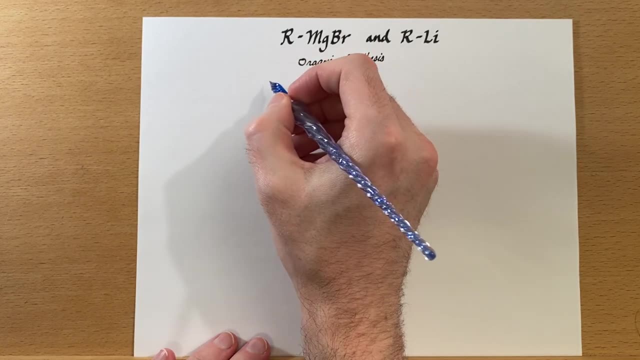 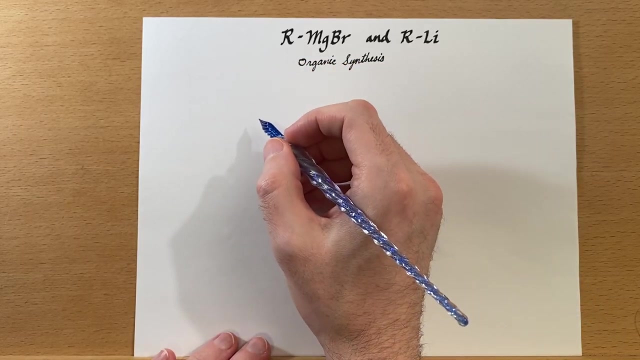 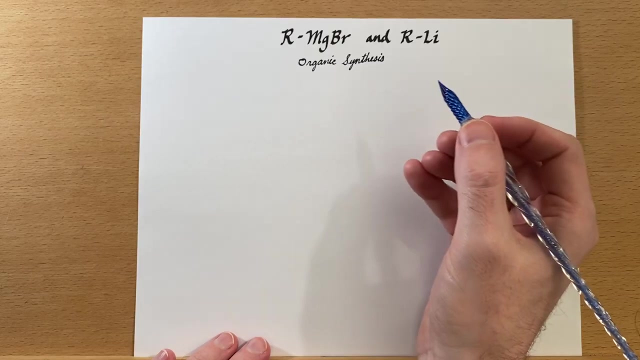 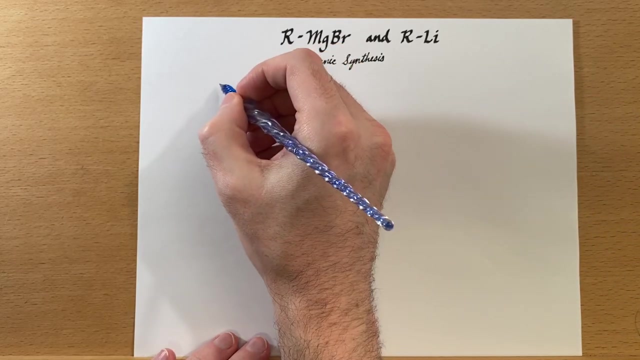 Furthermore, the reactions of these on carbonyls leave behind an alcohol, And alcohols are fairly versatile, So we can convert those into perhaps a bromide Using PBR3.. Or we could convert it into a tosylate or mesylate or one of those other excellent leaving groups using the tosylate chloride. 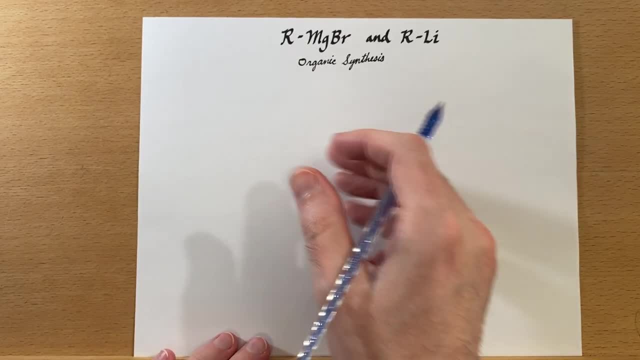 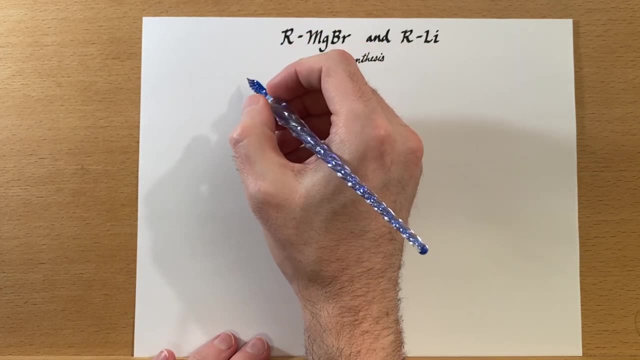 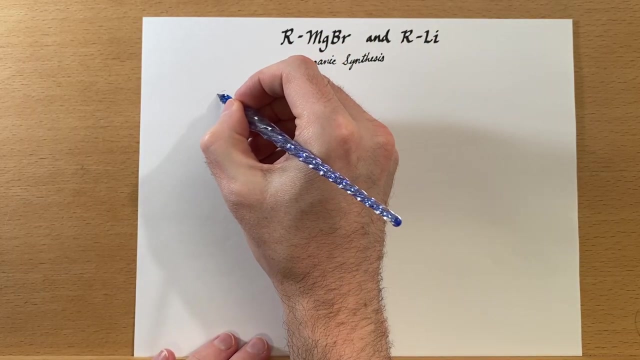 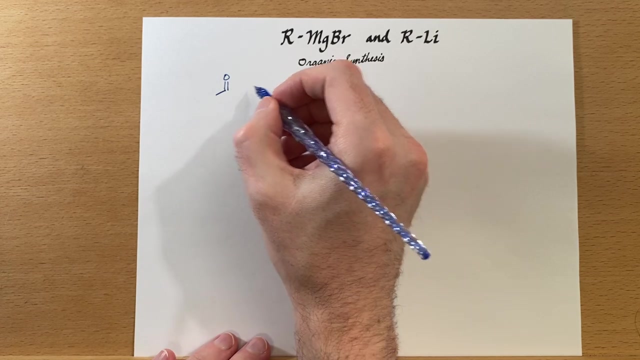 All of these allow us to continue the reaction forward after we've made an alcohol. We could even go a little bit further and just say, Well, let's start sketching out Just a possibility. here We can go from something that's like, say, an aldehyde. 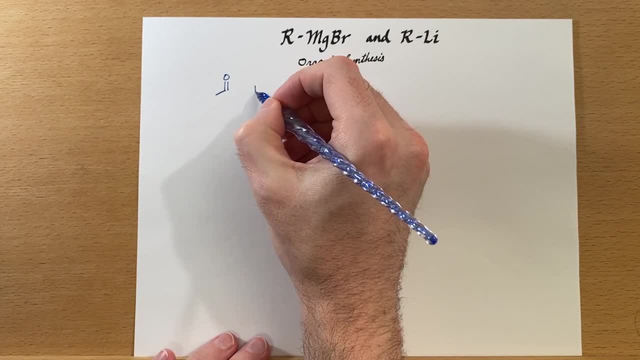 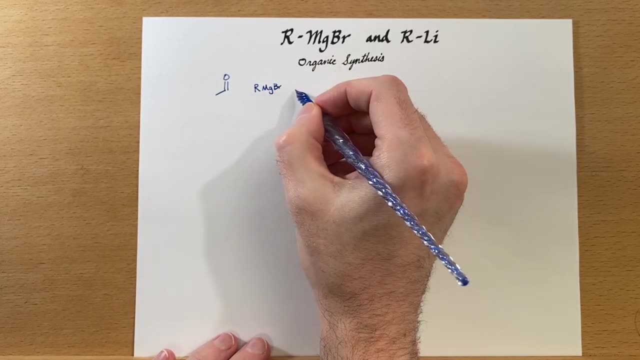 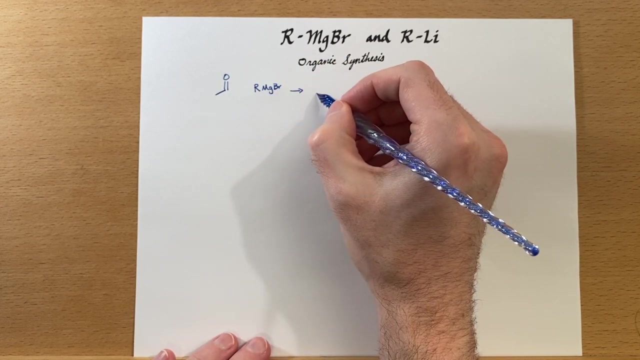 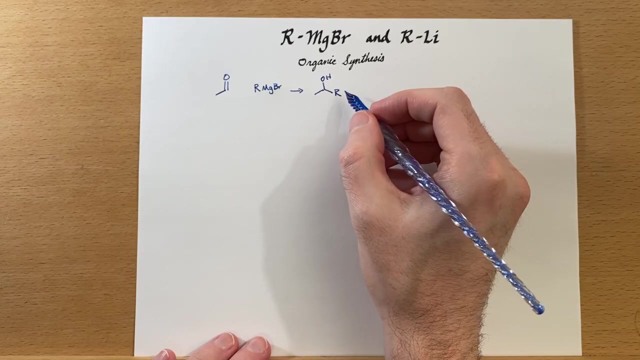 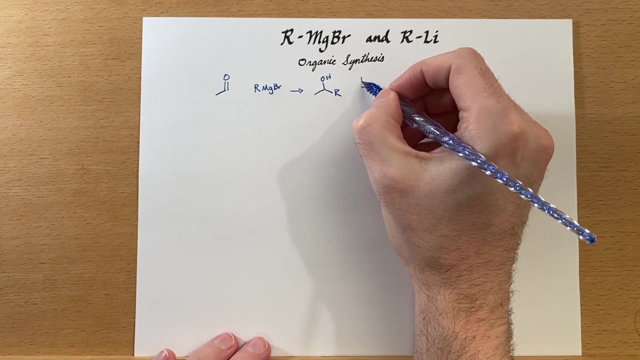 And then we could add a Grignard to it. This will generate an alcohol. In this case, since we started with an aldehyde, we generate a secondary alcohol. Put our R group there. Then from here, we could, just as an example, add PBR3. 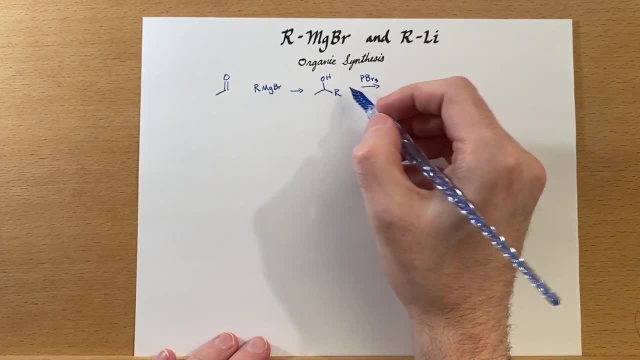 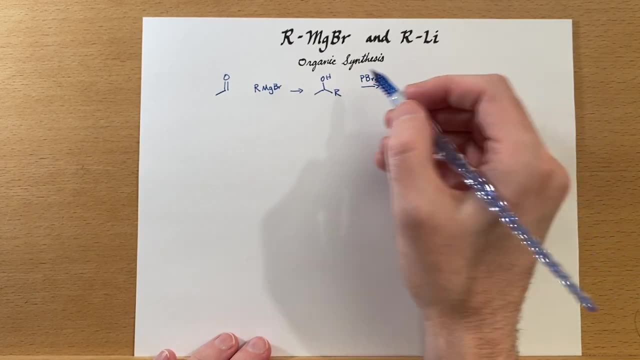 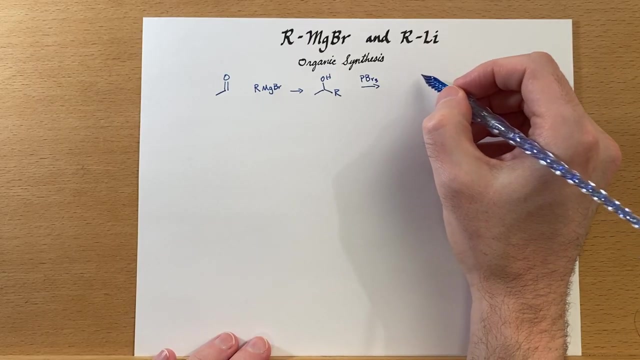 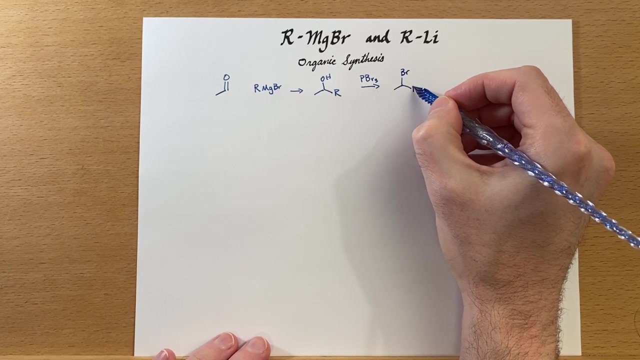 Or if there's no rearrangement and perhaps this is a simpler alcohol, we might be able to just add HBR with some sodium bromide and convert it to the bromide that way. But this is a little bit safer bet And we can turn it into the bromide. 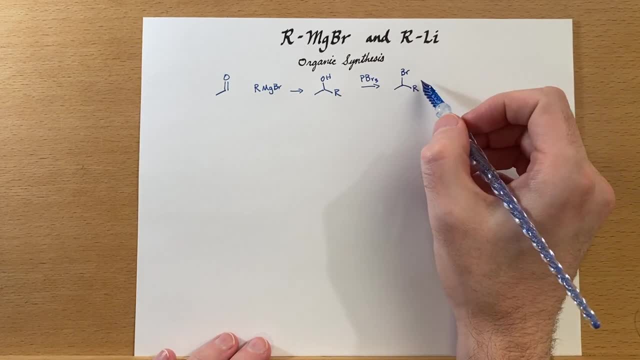 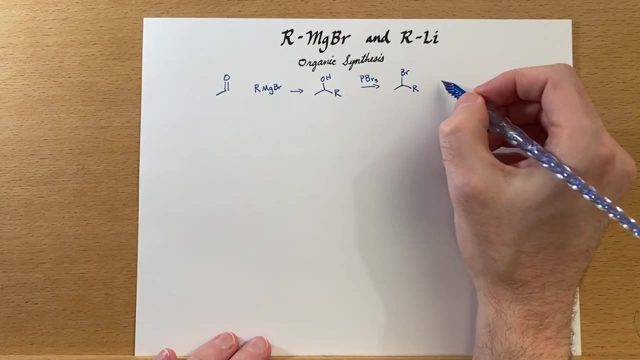 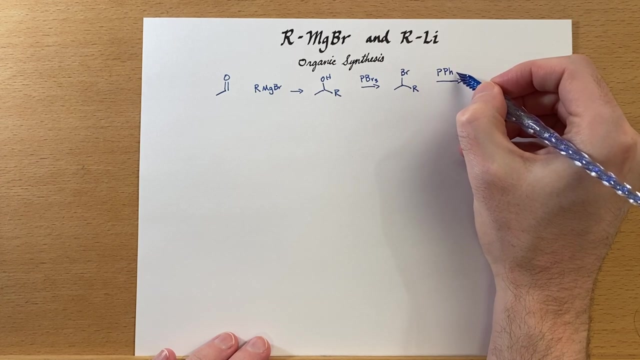 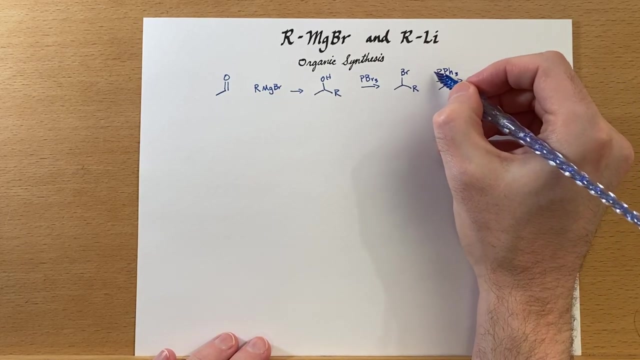 And we could either eliminate the bromide to form a double bond here, Or we could even convert this to the Wittig reagent, And we'll have to have some alkyl lithium stuff in here too, right, So step two there. 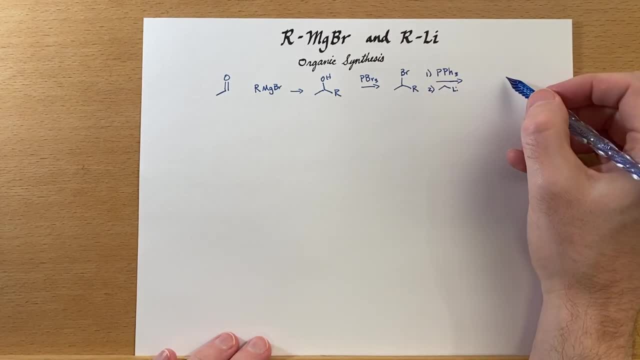 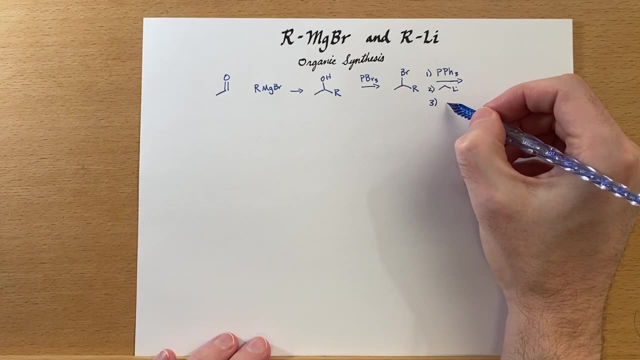 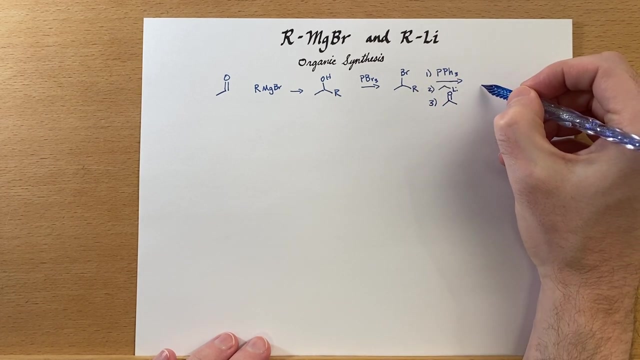 Make a Wittig reagent, And then we could react it with another. let's just say step three here. So it's all contained nicely, And we'll just add acetone to it, And then we would have this. So you can see how we can use this to really build up molecules. 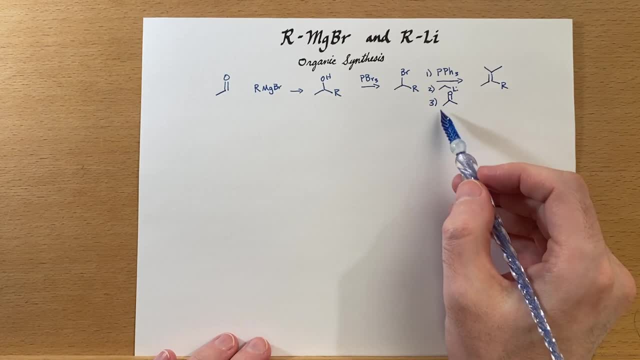 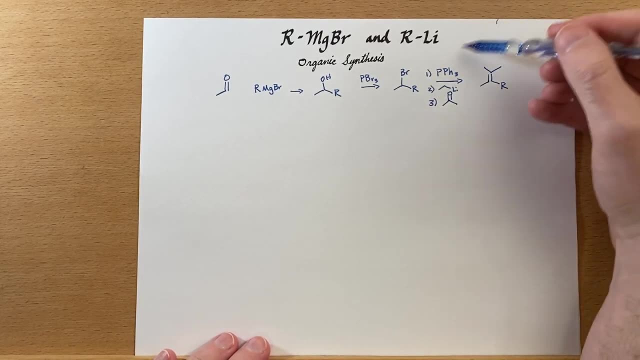 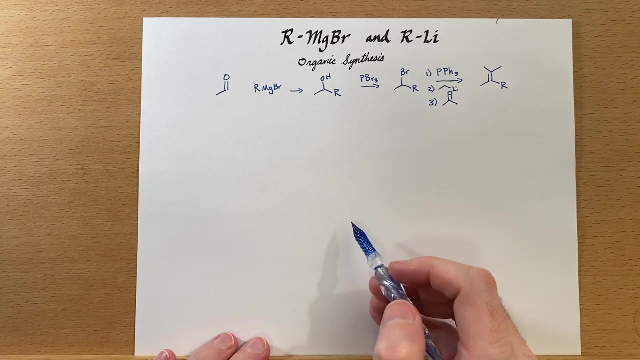 And of course, we could choose a more complicated molecule than just acetone And we could really start adding a lot of a large molecule up here together with whatever we put together down here, And you can start to see the versatility of all of the ways that we can go here. 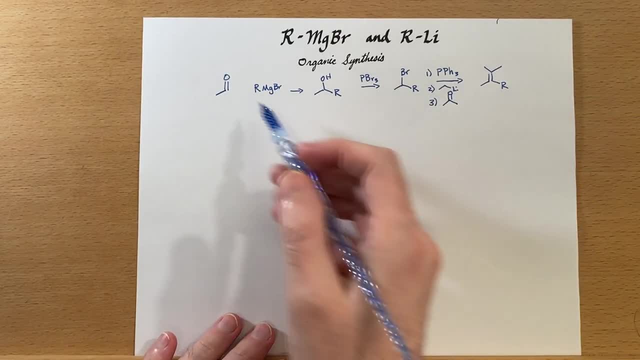 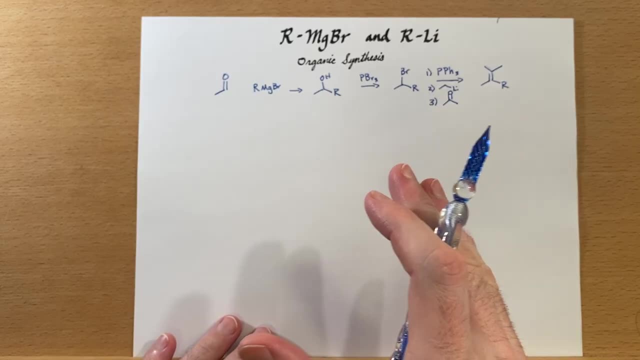 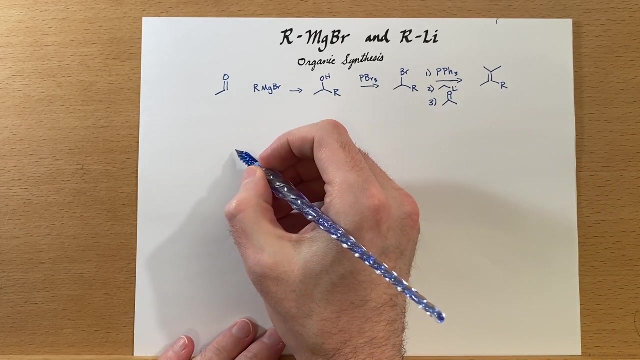 Let's take a little step back from just all the possibilities that we can do with an alcohol and converting and all of that to just look at the possibilities for just in the Grignard synthesis. So let's say we want to make a tertiary alcohol. 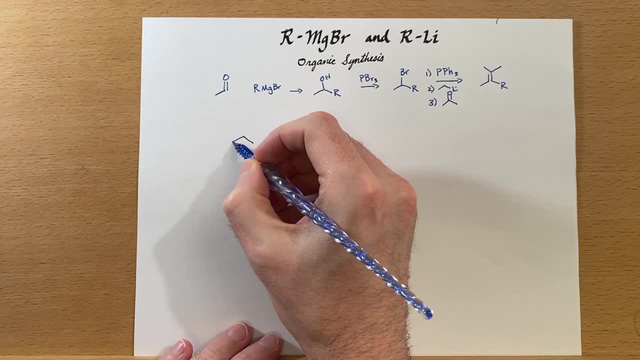 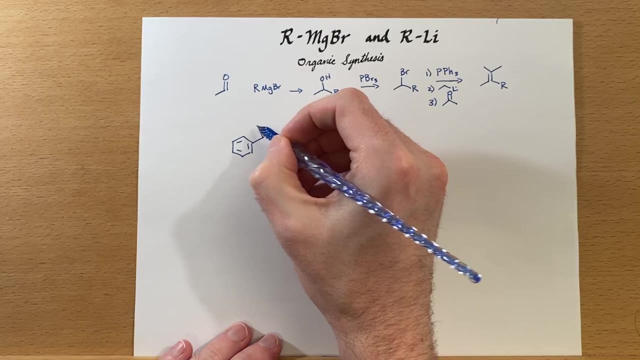 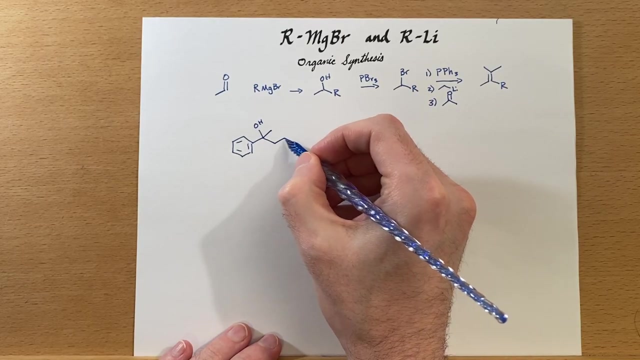 And It's got three different substituents on it. So we've got a benzene ring here And we've got an alcohol there, We've got a methyl group over here And then maybe a butyl group right here. Well, how could we make this? 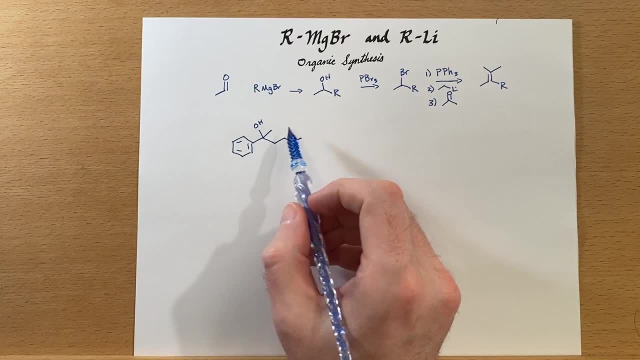 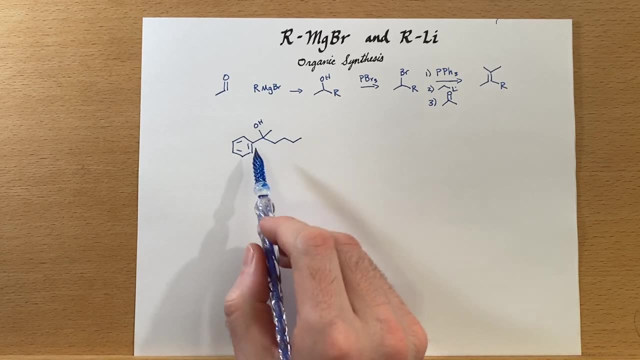 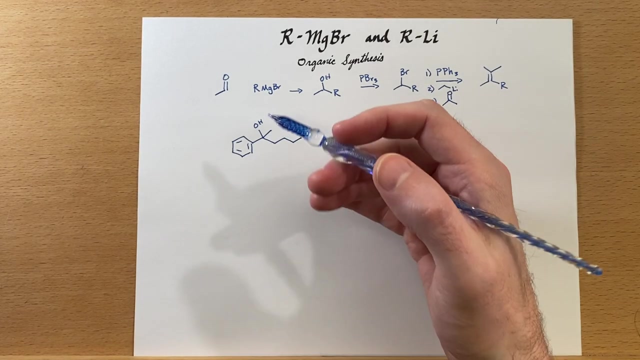 Well, when I see something like this, I'm looking at it and I'm saying, Hmm, that could have been a ketone. right Now, with a tertiary alcohol, I can think, Oh, ketone. And then I'm removing a Grignard or an organolithium- either one. 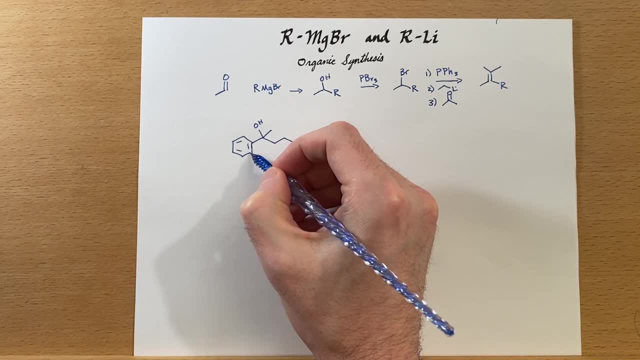 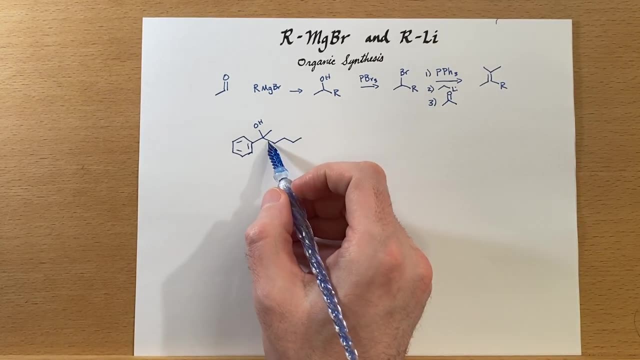 And I can think, Oh well, I just need to convert this back into the ketone. Now the question is: which one of these bonds should I break? Should I break this one, that one or that one? And the answer is: I could do it any one of those ways. 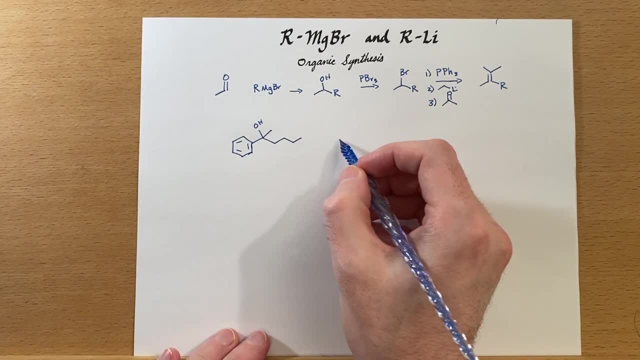 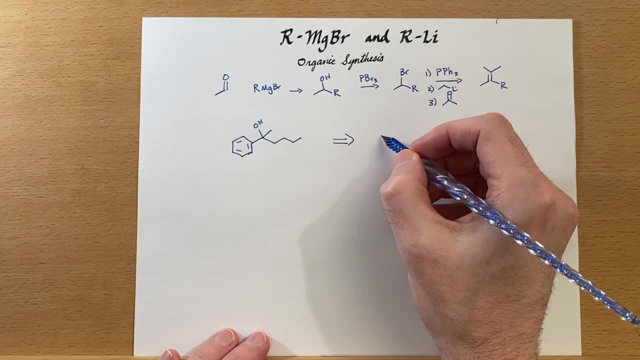 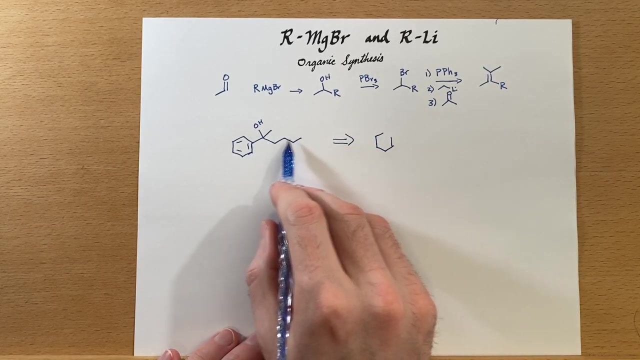 So let's see what could happen. I'm going to say we could make this from well, acetophenone, right. So let's say I break this bond right here And that's going to be my Grignard reagent. 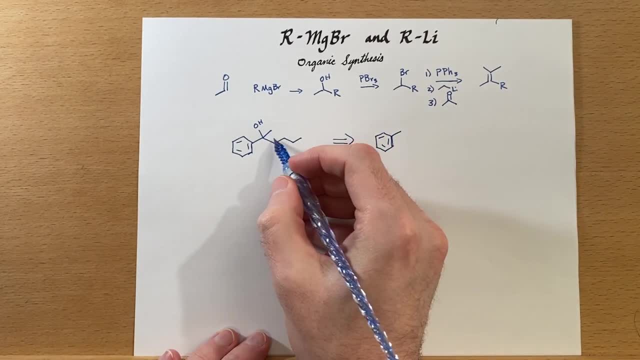 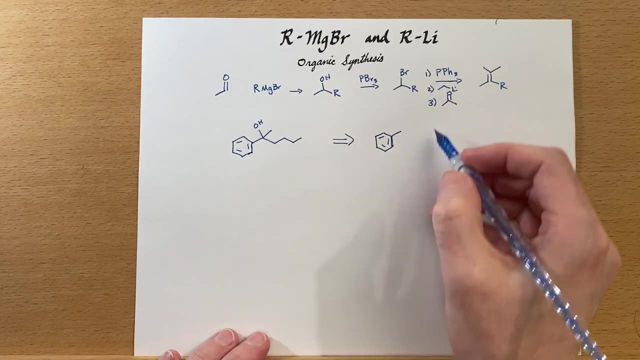 So I would start off. I break that. I put the double bond right here And I'm going to be left with a creatine. I'm going to put a carbonyl here, a methyl group there, a phenyl group here. 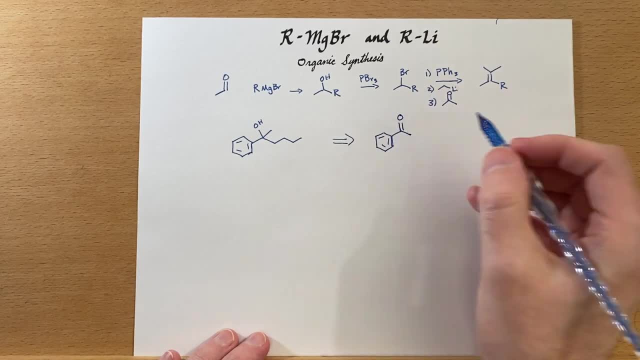 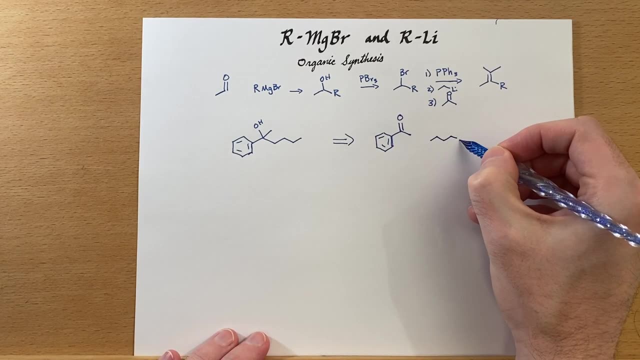 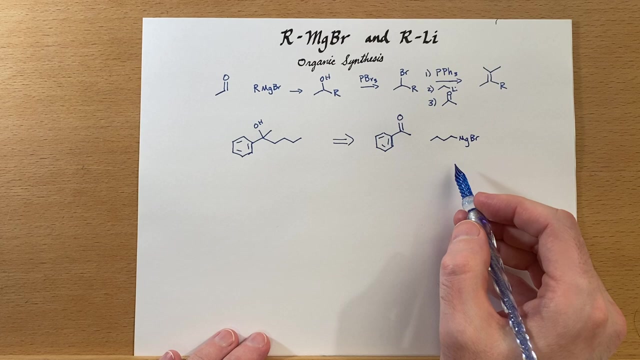 So I'm going to put a methyl group there, carbonyl here, And then I need my Grignard reagent, So it could be made from these two reagents And if we were to write this in the forward direction, we would also need to include an acid workup step. 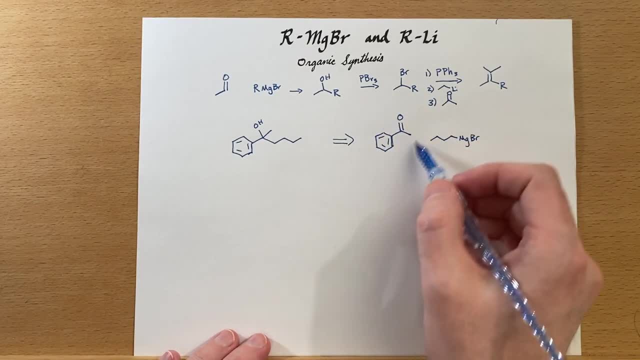 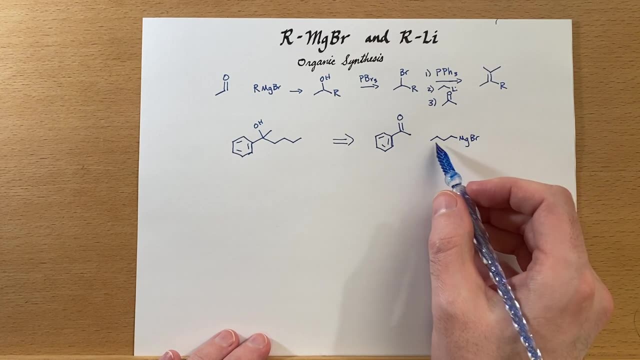 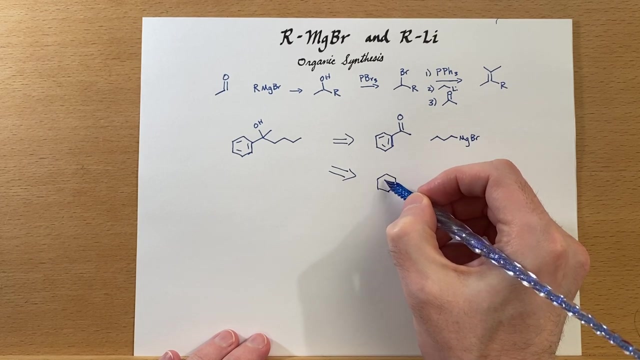 Just suffice it to say we could make it from this particular key tone, acetophenone, and that Grignard, which would be butyl magnesium bromide. Well, that's one of the possibilities. There's another possibility: We could instead construct this from the other, a different ketone. 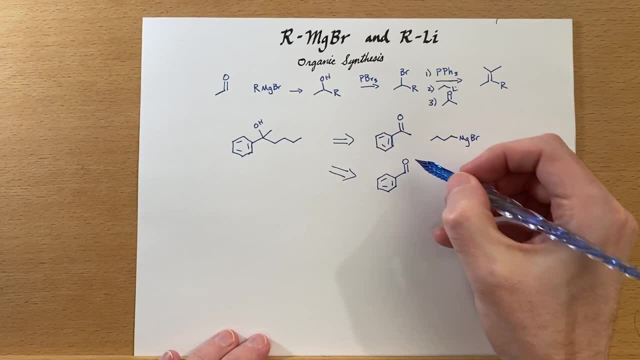 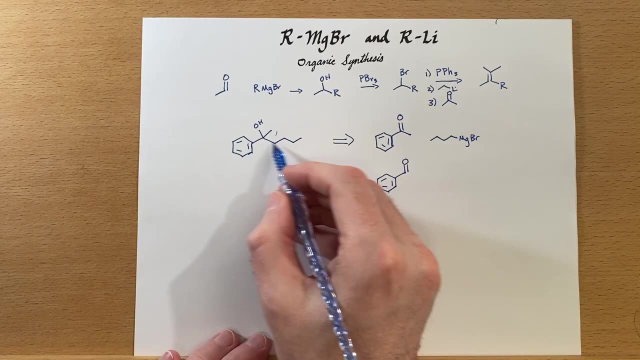 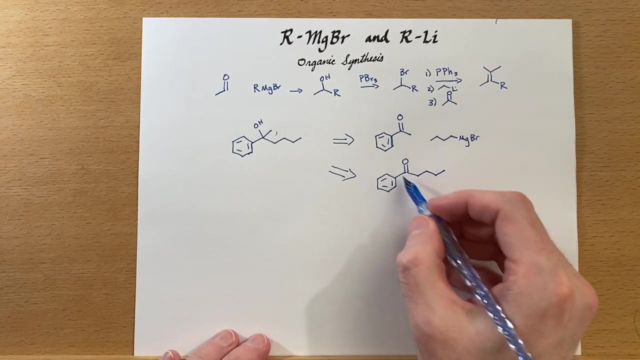 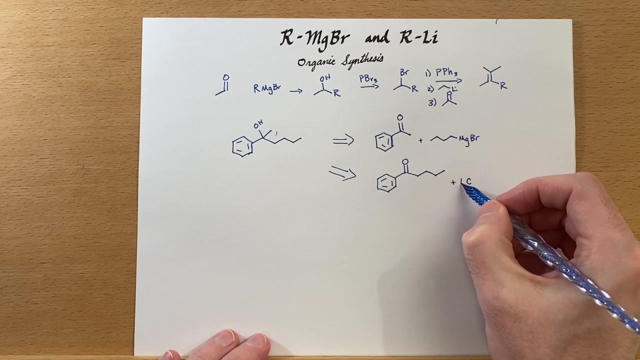 We'll still keep the benzene Benzene ring here, But now let's have the methyl group be the Grignard And this would be part of the original molecule here. So just like that. So if we have that, we can then change our Grignard to the to just a methyl group. 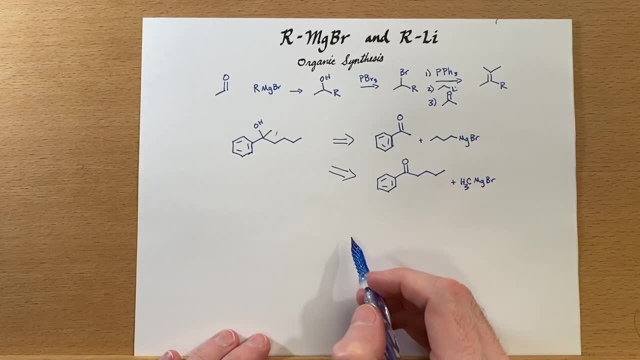 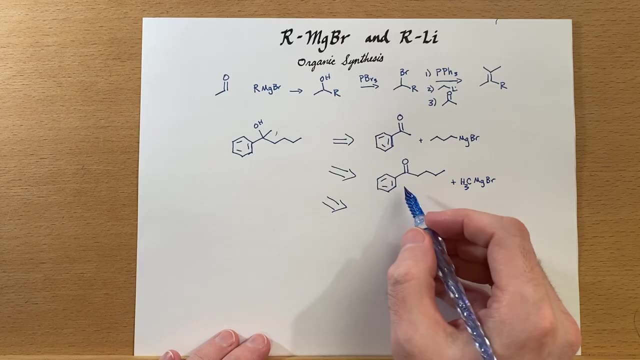 And if we do this, we can react these two together. We'll need an acid workup step. We'll make that product. Well, guess what? There's a third option to making this, Where the Grignard is now going to be the benzene ring. 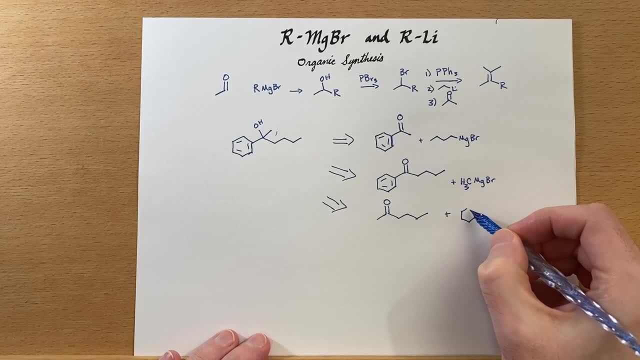 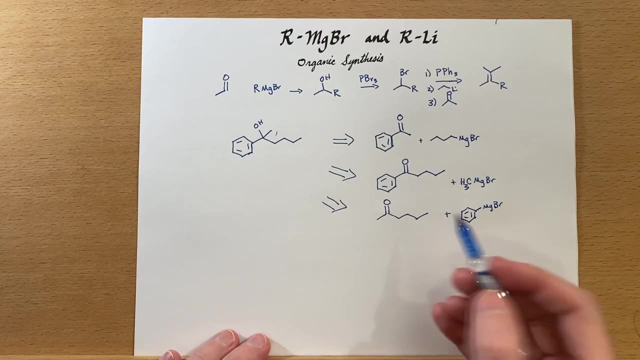 So phenyl magnesium bromide, Just like this, And again we'll need an acid workup step. All three of these particular reactions will make that product, And so you might be asking yourself: wow, how do I decide which combination to use? 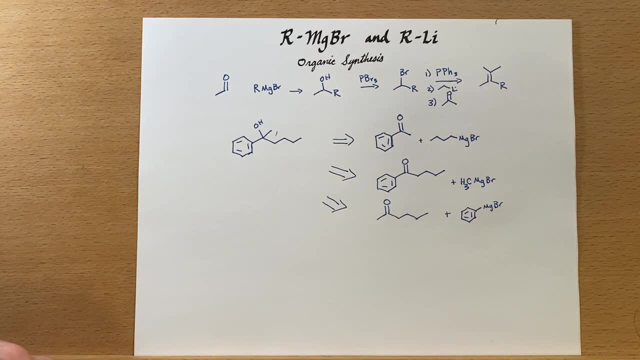 Well, without doing any experiments we won't really know which one would produce the highest yield. But if we were to do an experiment, we could figure that out And then we could decide: oh well, this particular combination produces the highest yield. 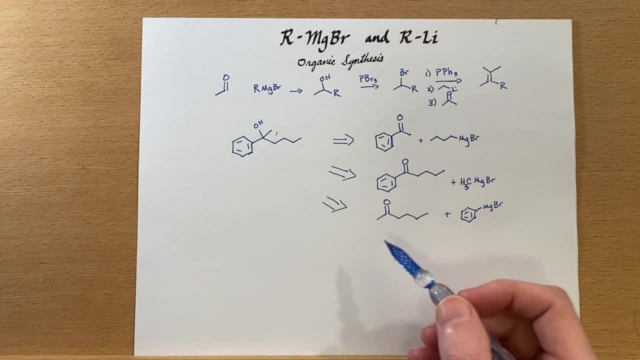 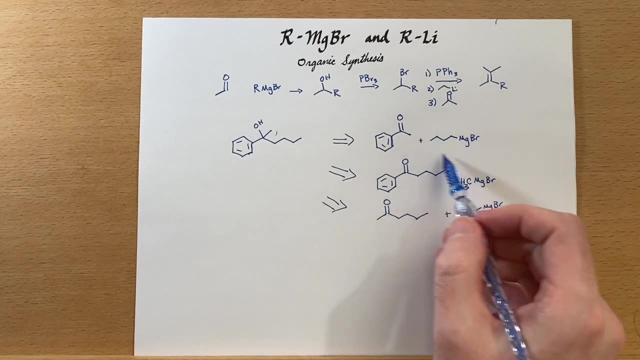 I'll go with that one. Otherwise you might ask yourself: oh, which one of these reagents do I have available? Which one of the bromides do I have? And if I have acetophenone in my stockroom? and I have acetophenone in my stockroom. 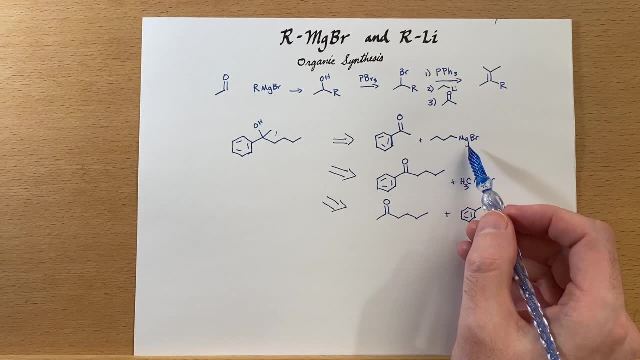 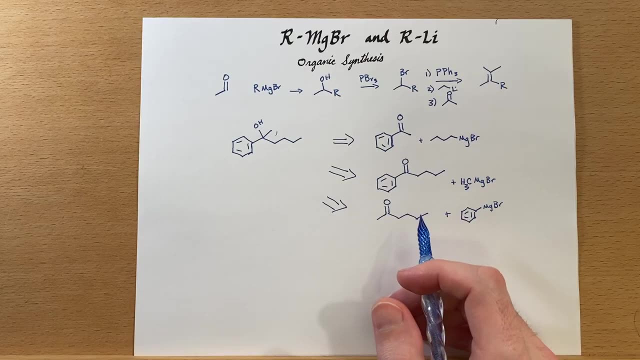 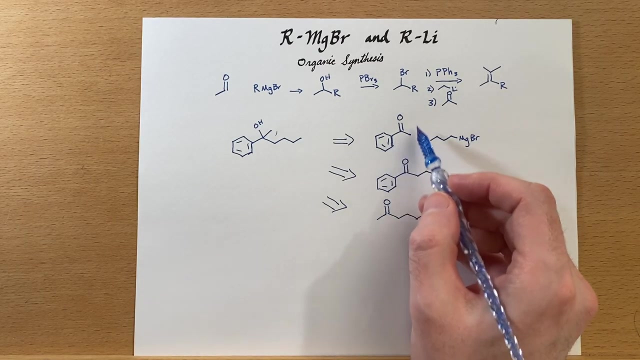 and I have one bromobutane and some magnesium, then I'll probably go with this route because I have those chemicals available. I may also check to see the price of these chemicals or just the availability to order if I need something. Personally, I would think that this first choice is probably the more available. 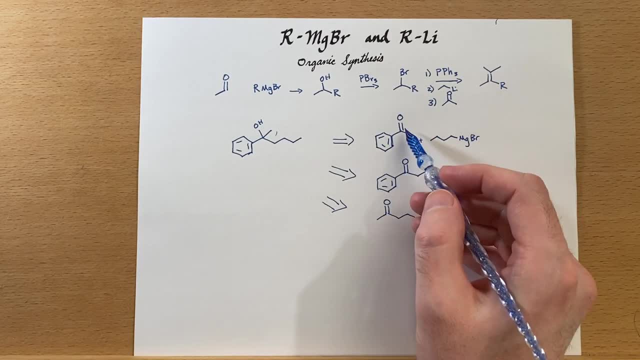 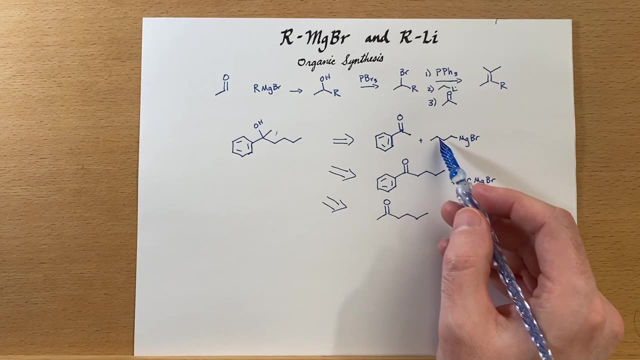 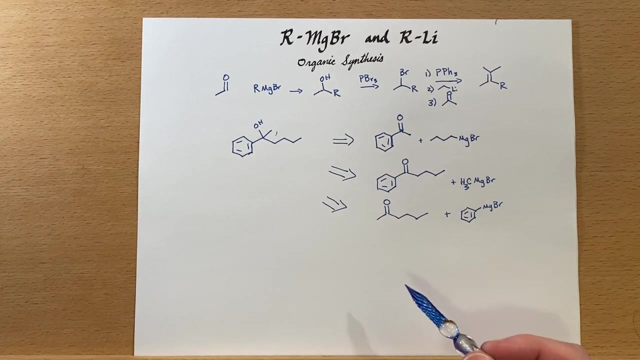 because acetophenone, that's a fairly common carbonyl or ketone and it's pretty common to have the one bromobutane as well. Also, I think these groups would be fairly easy to work with, But again, any one of these combinations would suffice.